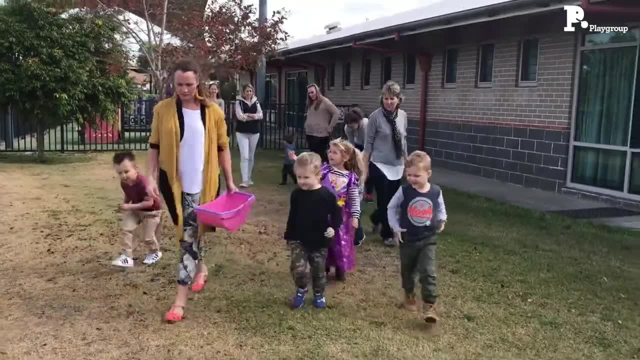 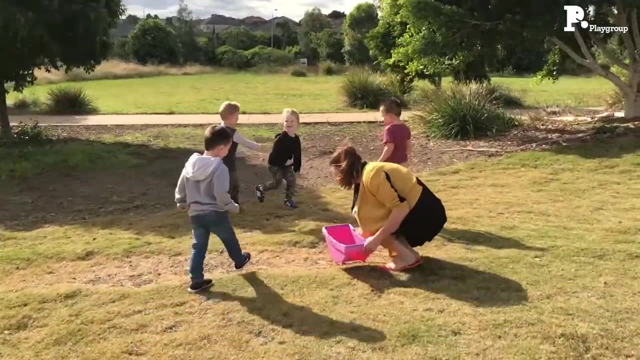 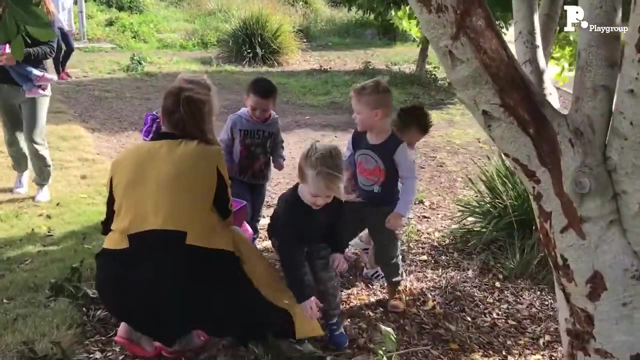 things are and why they're here and what use they have in the natural world, Like, for example, a seed grows trees or for example. But also these are our ultimate loose parts. They're free, they're everywhere. they're quite always very calming for children to be outside, And it means 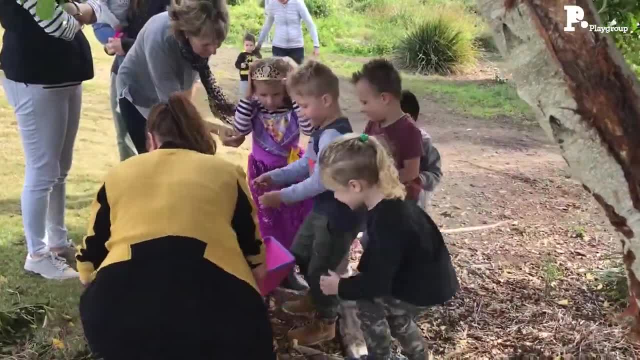 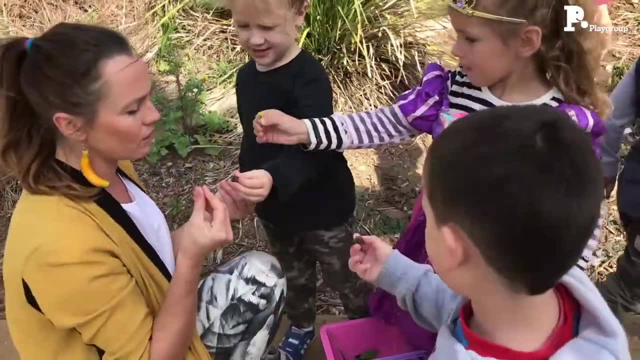 that when we use these materials for other things, when we come back inside or when we're building with them or making with them, they have ownership over these objects because they found them. It was intriguing and interesting to them already. So if we build and make using objects that they like, 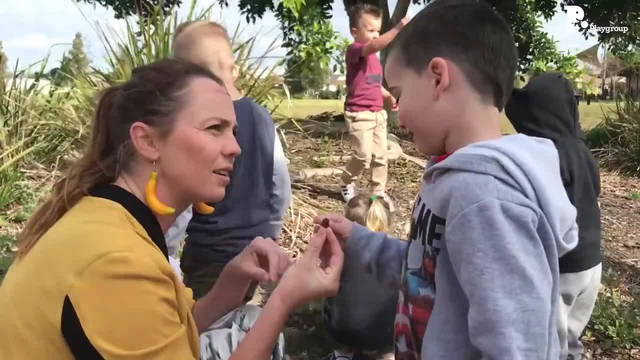 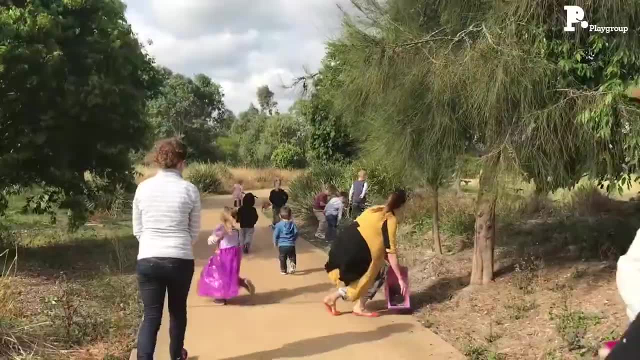 they're much more likely to be engaged. So, just going and collecting things that are interesting like little scientists out and about and then come back and have a look at them, I mean, you can sort them. you can talk about different colours, different shapes. which one is the? 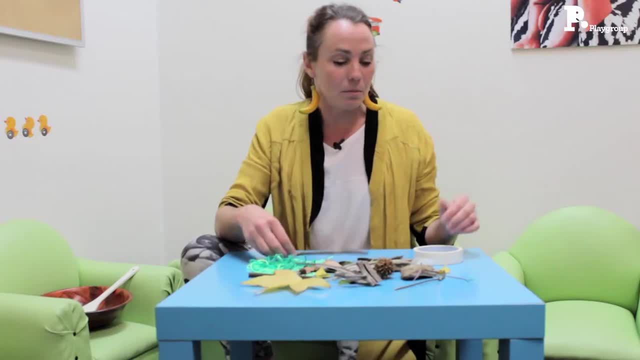 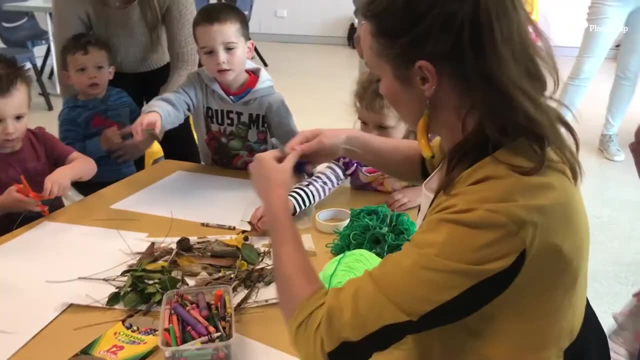 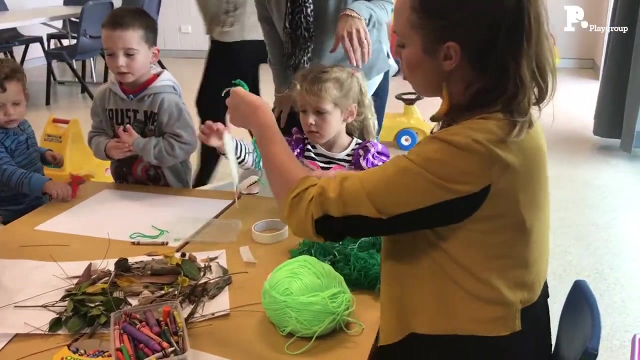 longest, which one is the shortest? And then, simply by adding a couple of simple materials, we can create all sorts of kind of craft activities out of these materials. So I've got some wool and I've got some masking tape, So, for example, we might want to start tying things. 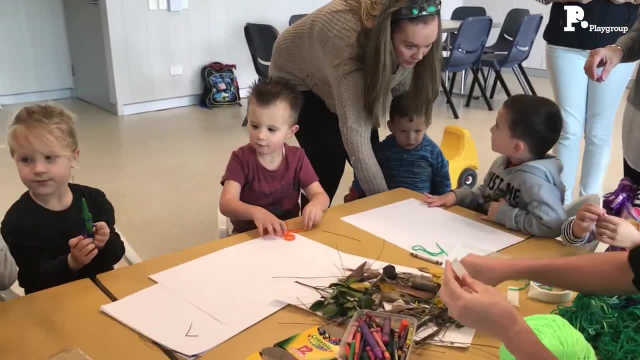 together And this is really important. So I've got some masking tape, And then I've got some wool and I've got some masking tape. So I've got some masking tape And this is really good for fine motor skills, for kids to practise tying together. I mean children nowadays don't even 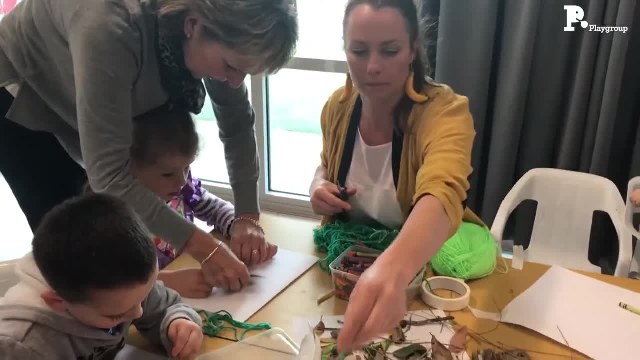 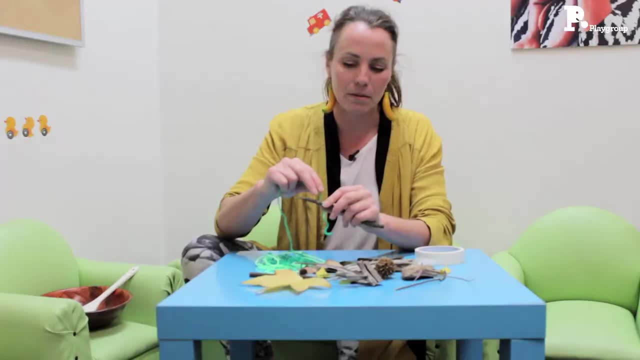 really get a chance to tie their shoes very often So they don't get that much time to really test out their fine motor skills with things like string. So it's really great for them to have that opportunity So we can practise just winding it around, We can practise tying knots. 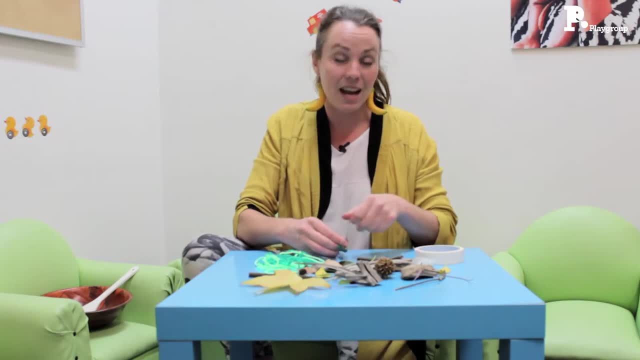 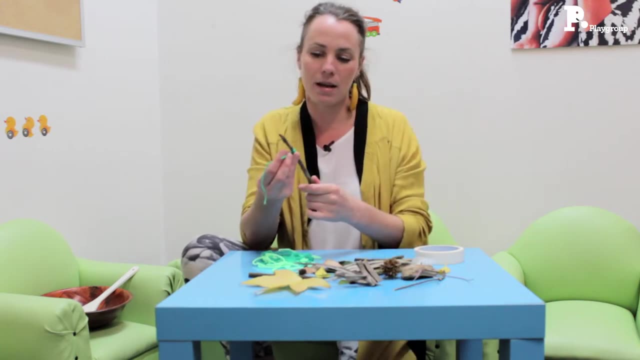 And we can even say: create a character. We could create a doll. you know, put a head on this. You know, this could be the head and it could be my character. Or maybe I could make a magic wand. Magic wands work quite well. So if we're going to make a magic, 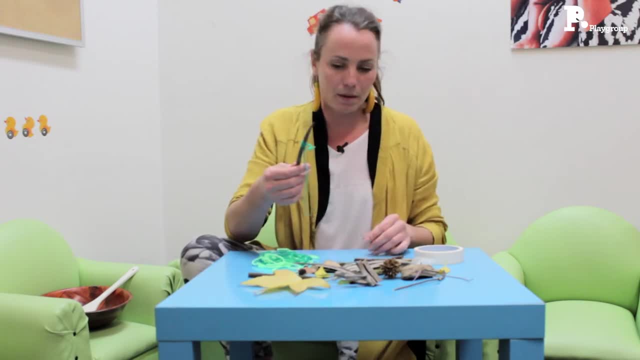 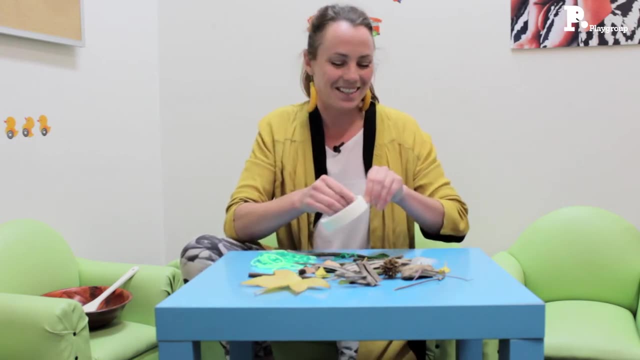 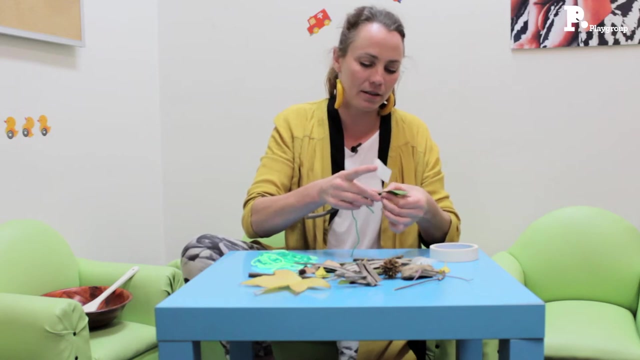 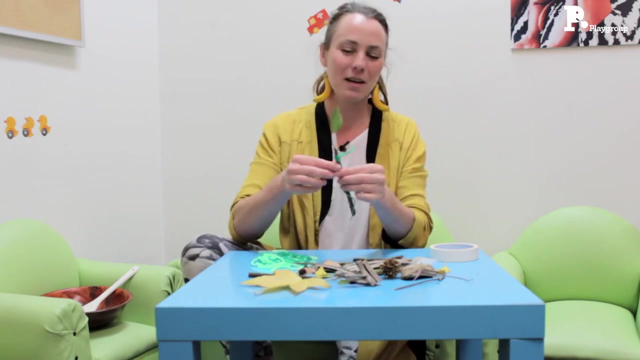 wand, just get a stick, and then maybe I'll attach some leaves to the top of it to give it the extra magic. So I'll just grab this tape here, get some masking tape, very simply wrapping it around the stalk of the leaf. Look, already it's one thing together and already this object has taken.